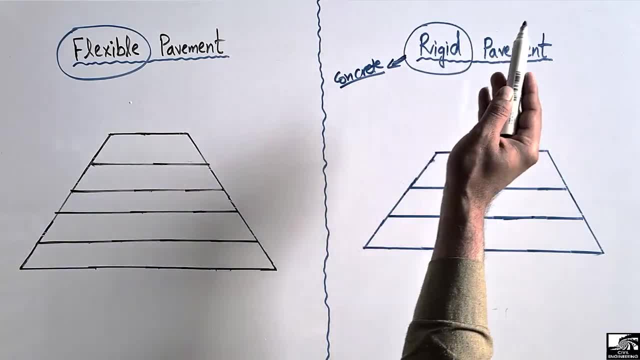 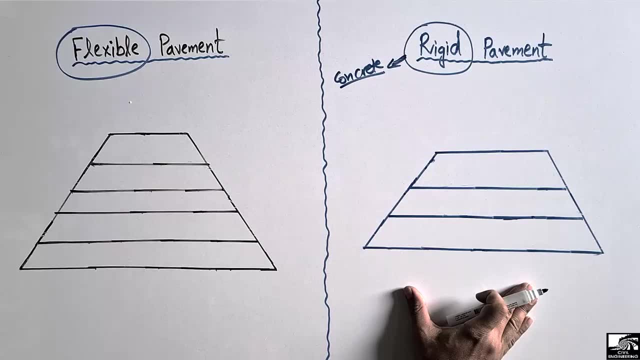 rigid pavement because it shows more rigid behavior to that of the flexible pavement. Now, what are the different layers in the construction of flexible pavement and the rigid pavement? So first we start from the flexible pavement. So, in case of the flexible pavement, the natural subgrade at the bottom of this flexible pavement, That is a natural. 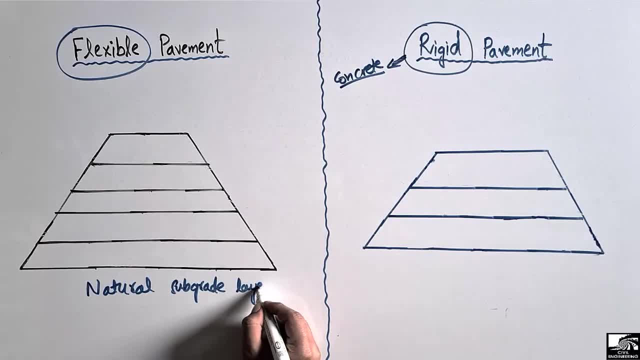 subgrade layer, And there is no such natural subgrade layer in case of the rigid pavement. On top of the natural subgrade layer, there is a compacted subgrade- Compacted subgrade layer, And this layer has been compacted to a certain level in response to the soft pavement. 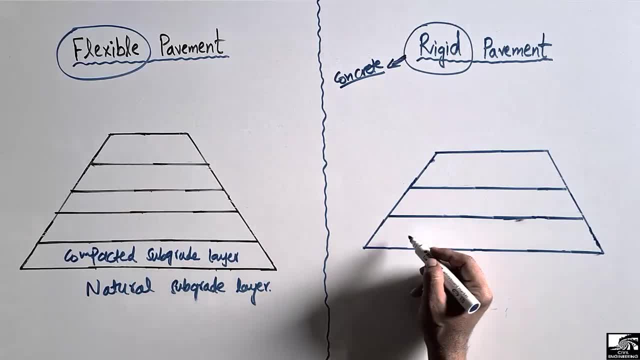 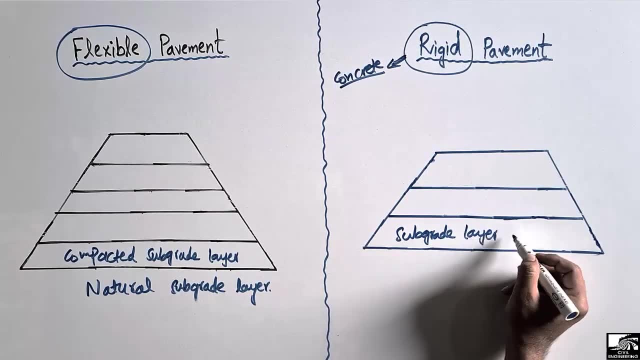 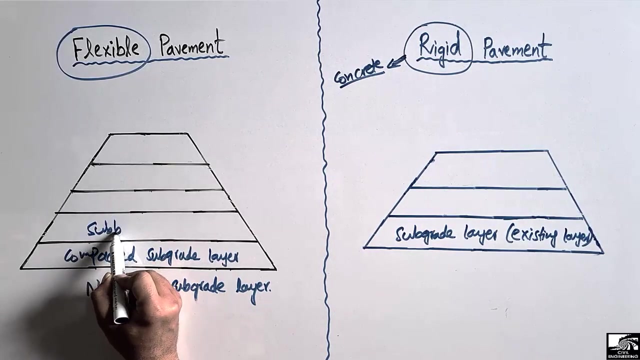 order to have certain degree of compaction- one in case of the rigid pavement- we also have subgrade layer, and this layer may be an existing layer, depending on the condition of the site. now, on top of the compacted subgrade layer, we provide sub base course- in case of the flexible pavement, sub base course. 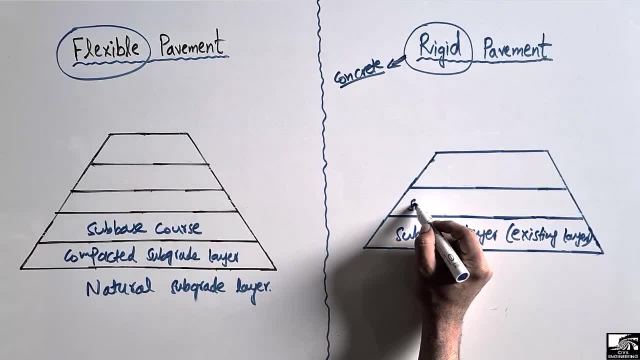 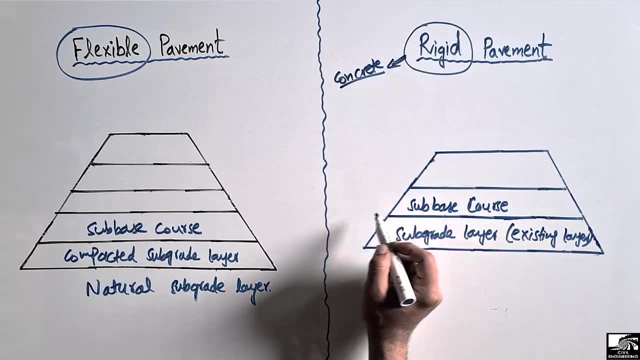 and also in the rigid pavement, there is a sub base course provided on the top of the subgrade layer sub base course and this layer sub base course and this sub base course also known is the frost protection layer, also known is the frost protection layer, because this layer is provided in order to resist the 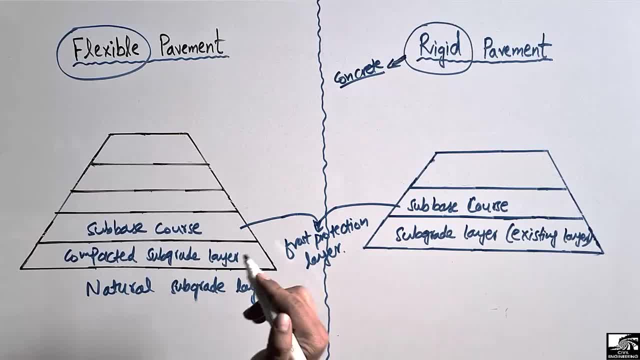 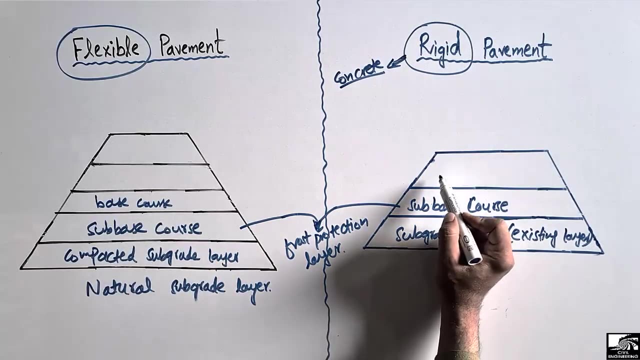 formation of the frost during the winter season. so this is mostly used in order to resist the formation of the frost On top of the sub-base cores. in case of the flexible pavement, we provide the base cores, While in case of the rigid pavement, we also have base cores. 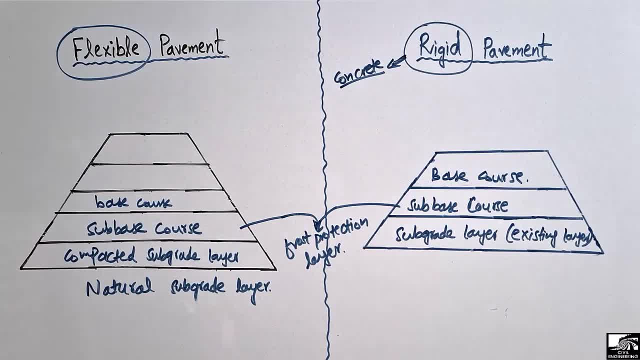 material in case of the rigid pavement. Now, these three layers are mostly same in both types of the pavement, While in case of the flexible pavement, on top of the base cores, we provide certain type of the coating known as the prime coat. This type of coating is known. 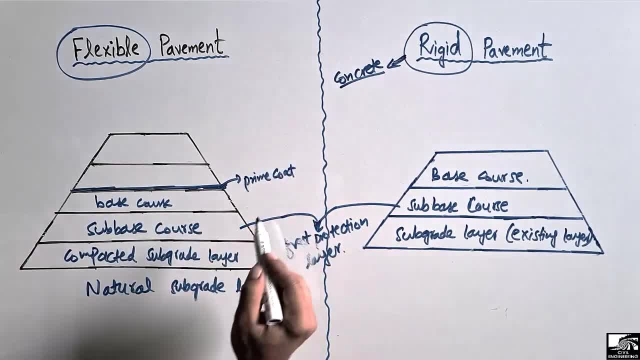 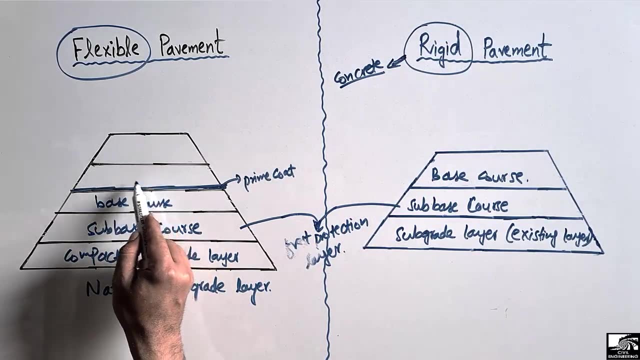 as the prime coat, and it is usually made up of bitumen material. So we provide the prime coat on top of the base cores in order to resist the penetration of the rainwater inside into the other layers. So, and then on the top of the base cores, we have another layer which is 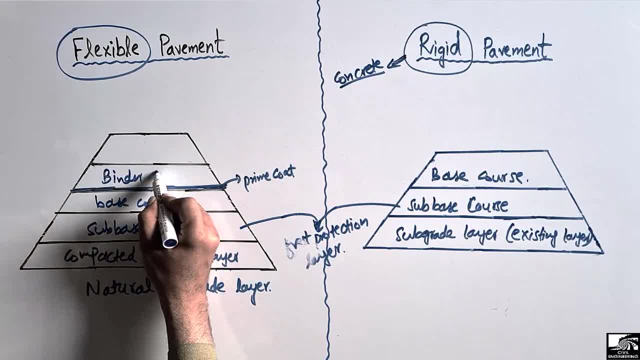 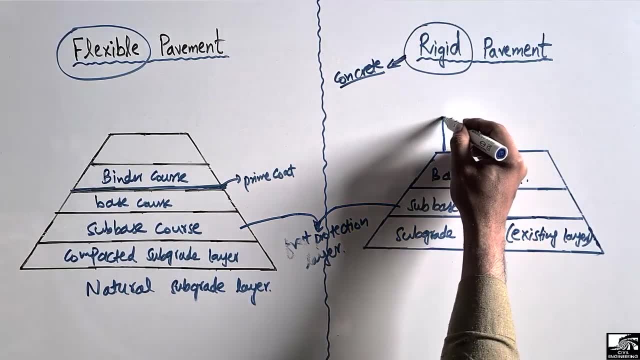 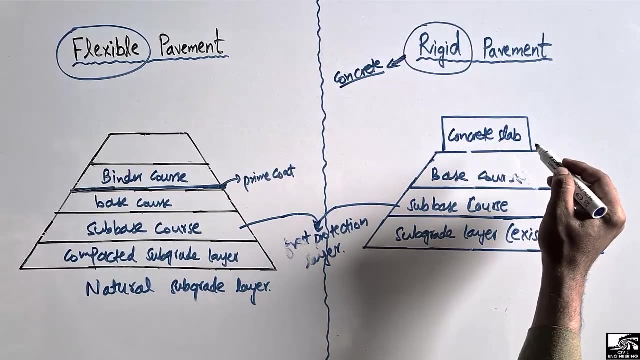 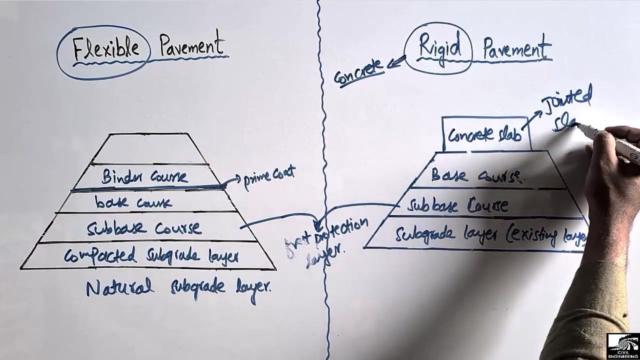 called as the binder, Of course, while in case of the base cores, on top of the base cores, we provide concrete slab, Concrete slab, And this concrete slab is a jointed slab. What it means? It means that we provide two types of the joints. 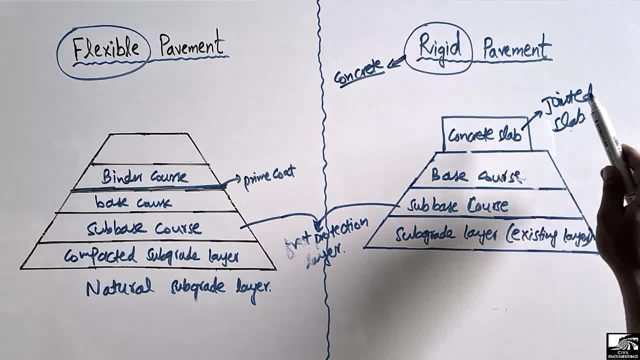 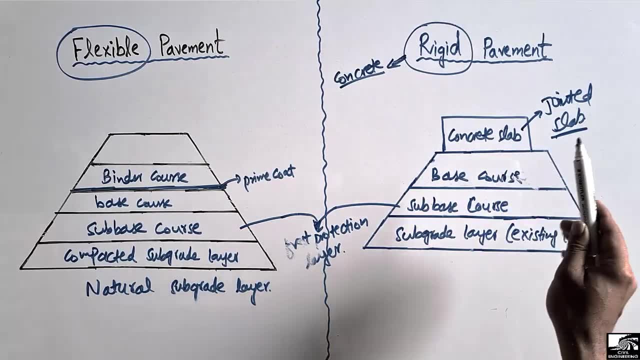 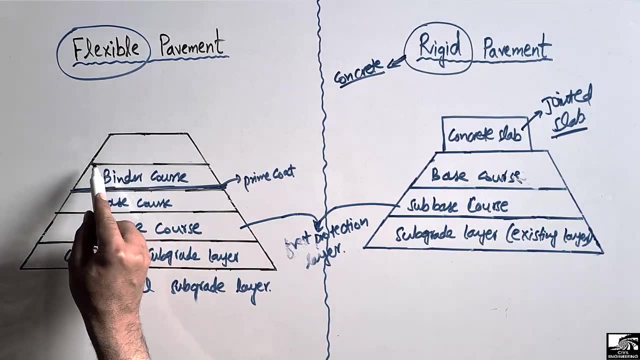 There is transverse joint and the longitudinal joint, and these joints are provided in the slab in order to resist the thermal stresses created due to the temperature variation in the slab. Now on top, here in case of the flexible pavement on top of the binder, 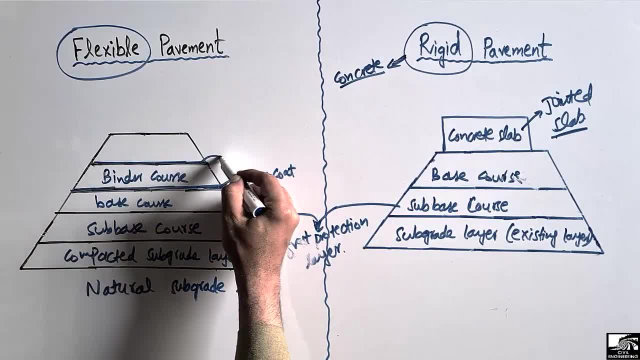 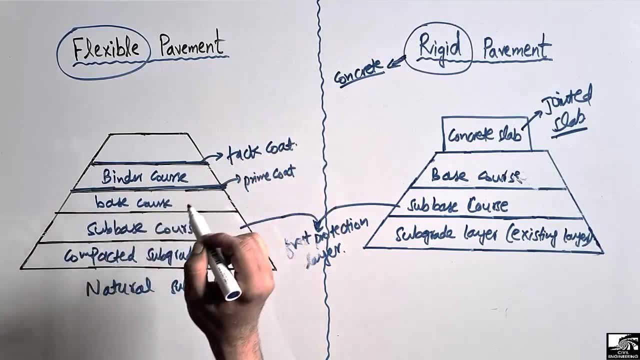 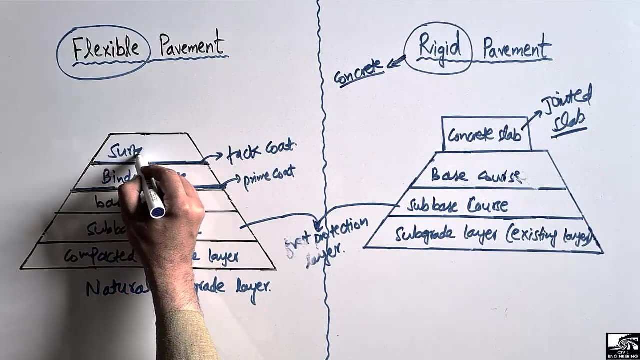 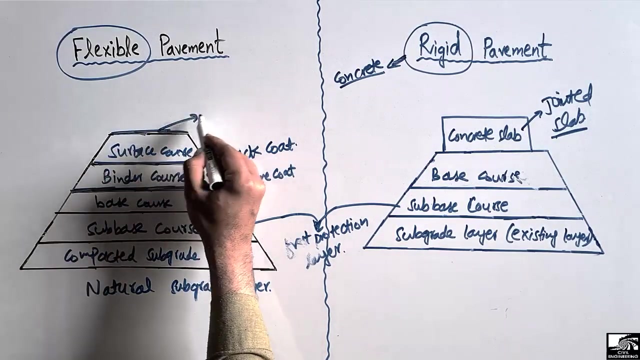 cores. we provide another type of the coating, which is known as the take coat, Take coat and on top of the take coat we provide the Corded Coast Coat, provide the top surface and this is known as the surface course. and on top of the surface course, we provide another type of coating, which is known as the 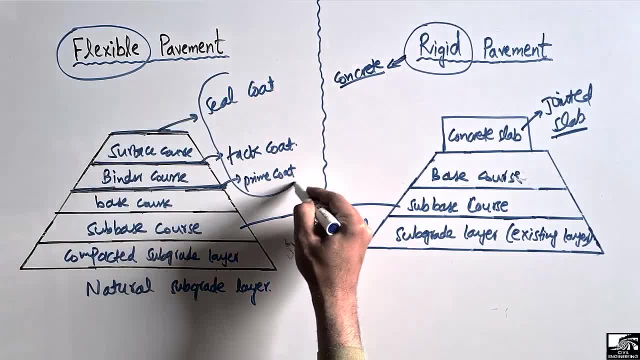 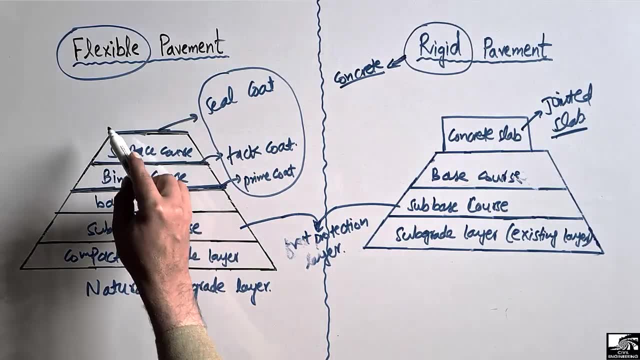 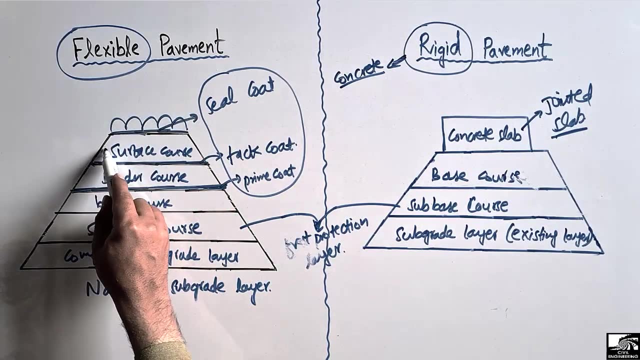 seal coat, and this three types of the coats are used to prevent the penetration of the rainwater into the lower layers. so when the load X on the top of the surface course, the load will be transferred from to the surface course and then to the binder course, and then to the base course and into the sub base. 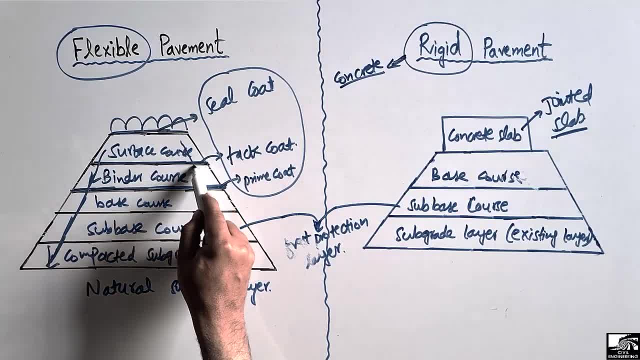 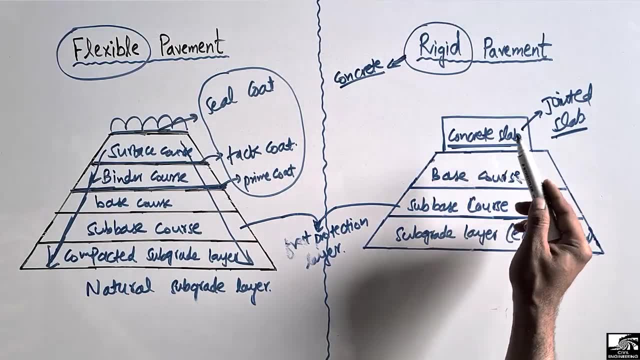 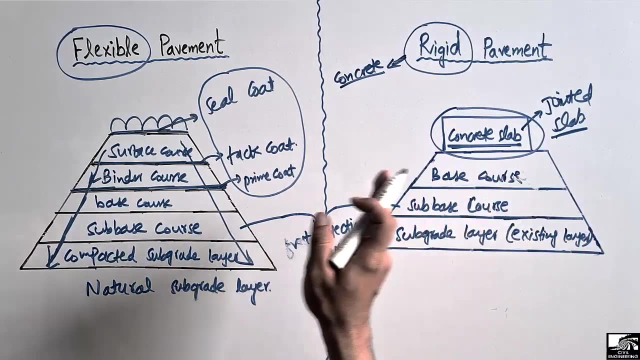 and then to the compacted subgrade layer. so load transfer in this way from top to the bottom. similarly, in this way in the case of the concrete slip, the mostly the most load is taken by the concrete slip and it does not show the same transfer mechanism like the flexible pavement, but it shows the mechanism of the flexure. so 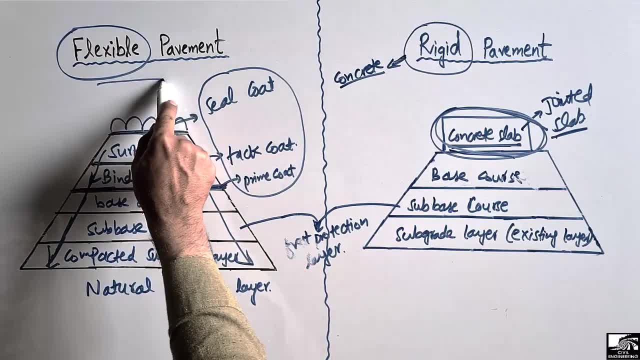 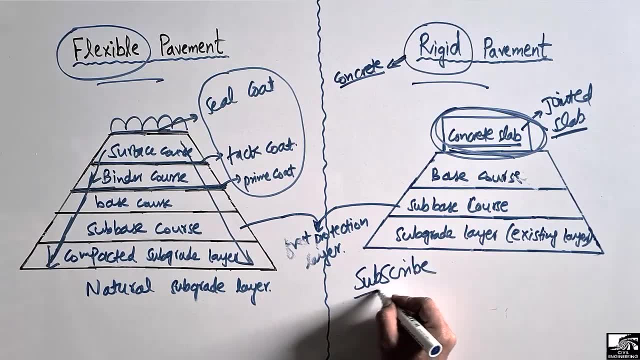 these were the different layers in the construction: the flexible payment and rigid payment. hope you guys understand and don't forget to subscribe our channel for daily seven engineering videos. thank you for watching our video.